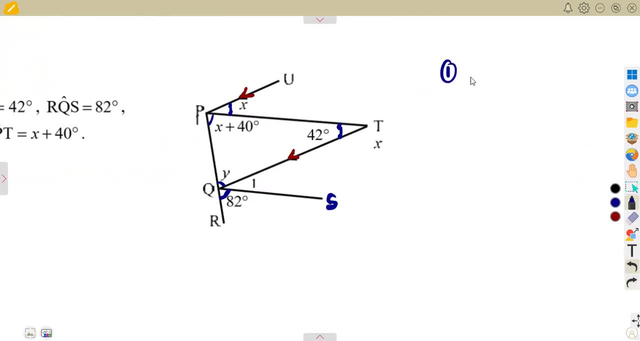 So how can we prove that? That is the question. Prove that PT is parallel to QS. How is that possible? As long you are working with parallel lines in order for you to prove, you are supposed to think of your alternate angles, the ones that gives us a Z. Think of the. 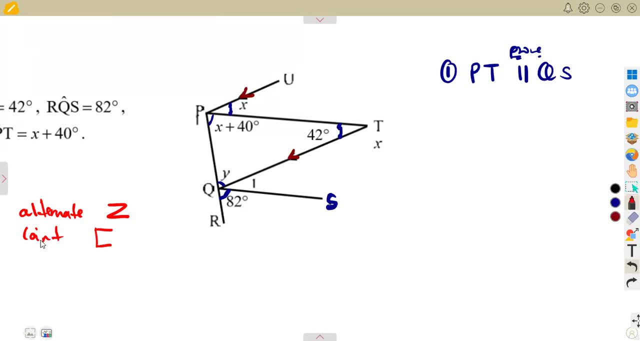 interior angles, the ones that gives us that C. Think of the corresponding angles, the ones that gives us F. All this part, you're supposed to be thinking about this. If it can satisfy one of these, if the conditions can satisfy one of these, therefore, those lines are parallel, So we have to. 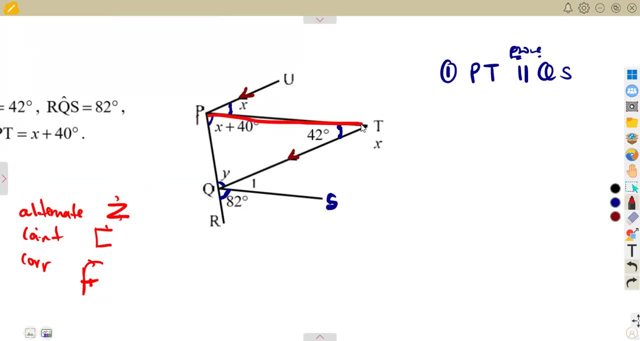 figure out. We are focusing on line PT and line PS. Is there any angle that we can calculate or that we can have? That is the question. Is there any angle that we can calculate or that we can have? All right, We are given that these two lines are parallel, So it follows that angle X is equal to. 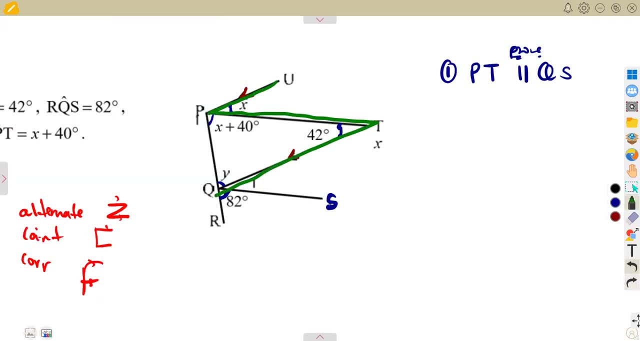 42 degrees. We are forming a Z today- Alternate angles, So X is equal to 42 degrees. So in this case we can see that our angle X is 42 degrees from alternate angles. All right, So these are alternate angles that we used there. 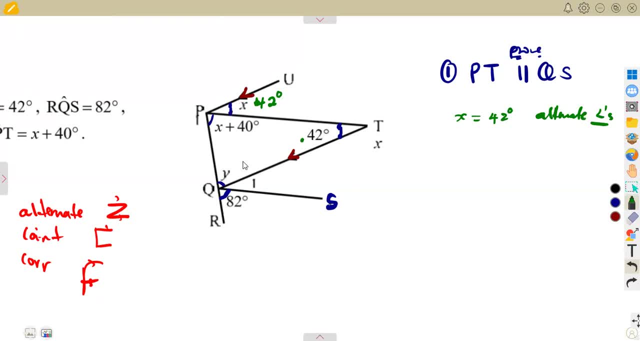 this angle and this angle forming a Z By having this angle X, it means where there is given X plus 40. But which is angle Q, P, T is given as X plus 40 degrees And our X is 42 degrees, So we're just. 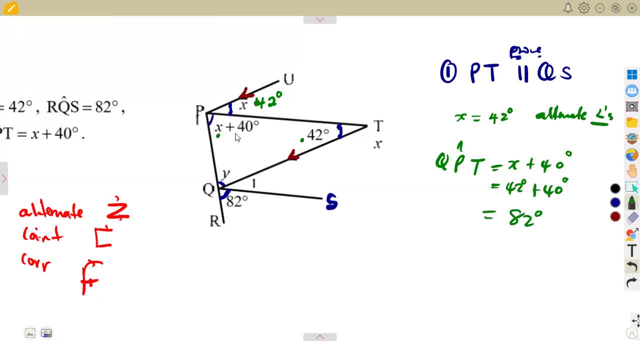 going to substitute that and add, which is 82 degrees. So the wall of this angle that we are seeing here can be written numerically as 82 degrees instead of that algebraic expression that was given. There is something that is happening here. I want us to consider this. 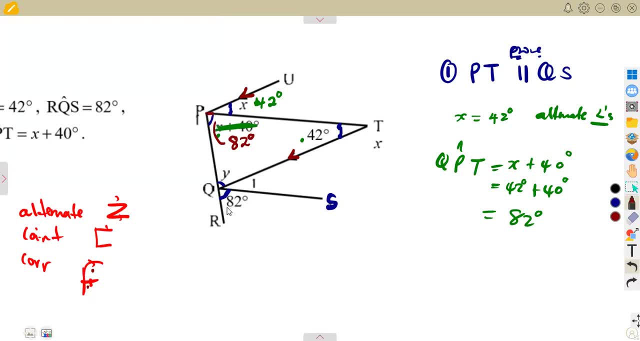 We are forming 82 degrees, 82 degrees and F there, If you check properly, Here that's an F, this one All right. We are forming an F, Angle of 82 here, angle of 82 here. So what does this tell us? These angles, these lines are parallel. 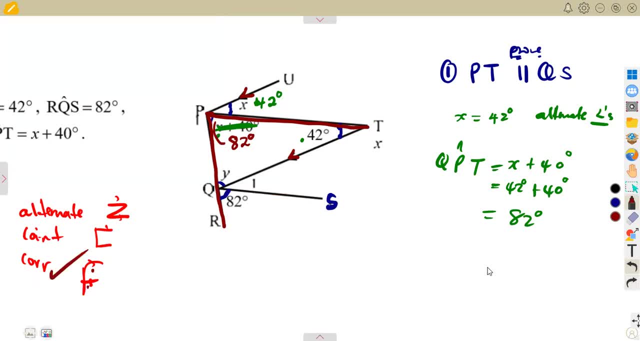 Why Corresponding angles? It can't be that of nature to say RQS, this angle, RQS is equal to the angle Q, P T that we calculated, which is 82 degrees. It cannot just happen like that. It means these two lines, they are parallel, P T is parallel to Q S. We are talking of what? 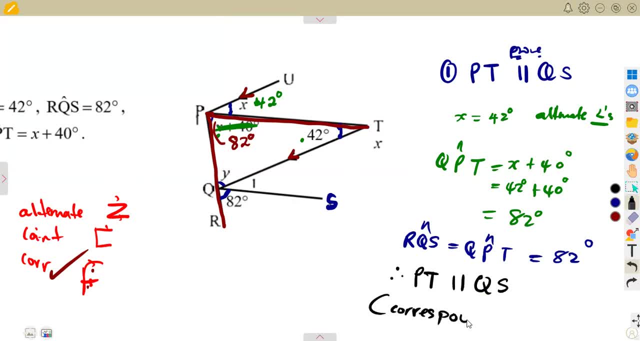 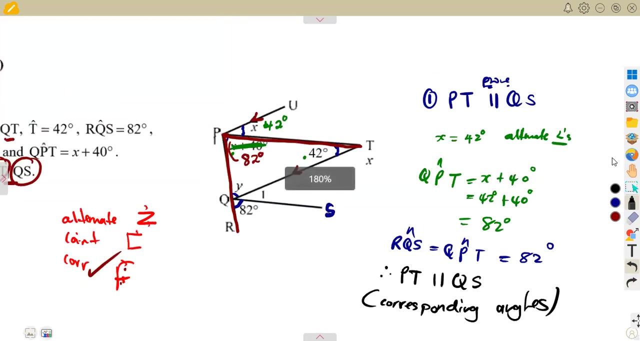 Corresponding Angles there, That is, corresponding angles. So, like I said before, you are not going to have corresponding angles. always Another part you prove maybe there was alternate angles. It depends on the situation that you have on that particular diagram. So that's why I was saying: do as many questions as possible. 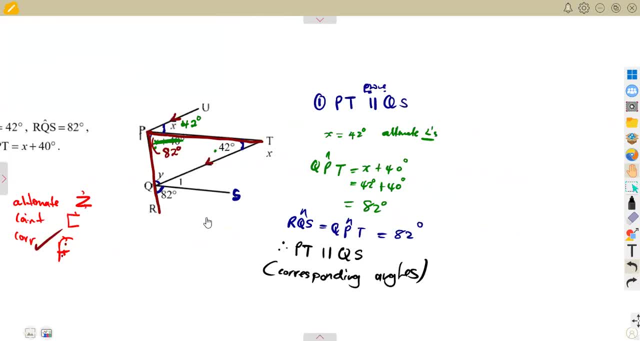 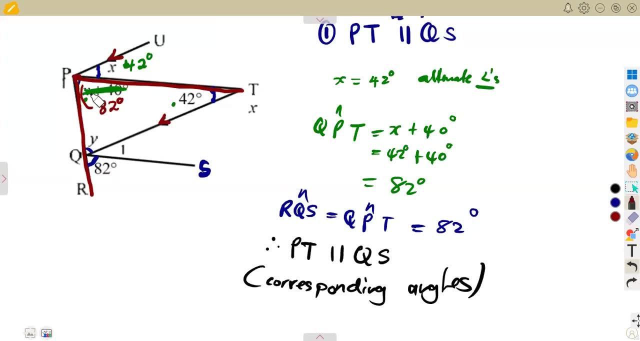 Calculate the value of Y, That is, calculate Y. in that case, How can we calculate the value of Y? All right, We have got this angle as 82. This one is 82. This one is 42. So what is it Angles? in a triangle, they add up to 180 degrees. 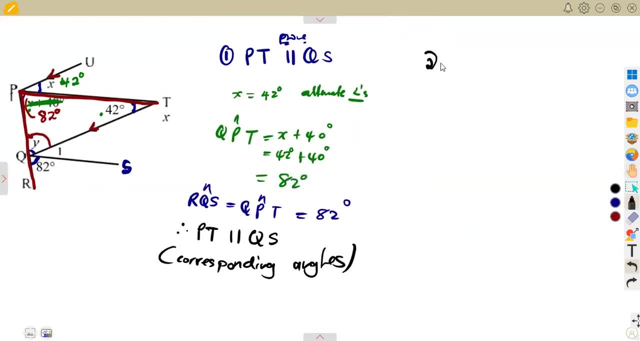 So you can calculate that Y from there, Just like that. All right. So number two, using angles in a triangle. from triangle P, Q, T. We know that angles in a triangle, they add up to 180 degrees. So if I am to add these angles, that means Y is going to be 180 degrees minus. 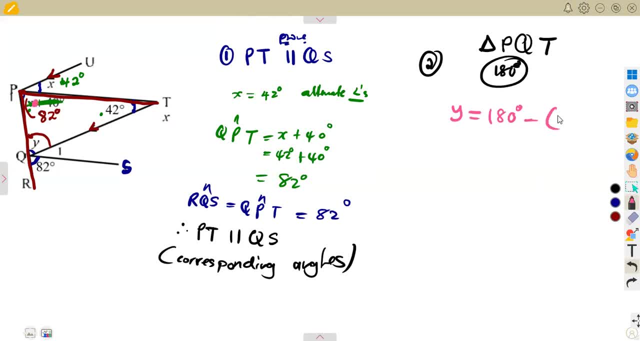 these angles that are inside of the triangle. There is an 82 degrees. There is also a 42 degrees inside of this triangle. Remember, if we were to add this one and this one, all these, they were going to give us 180 degrees.